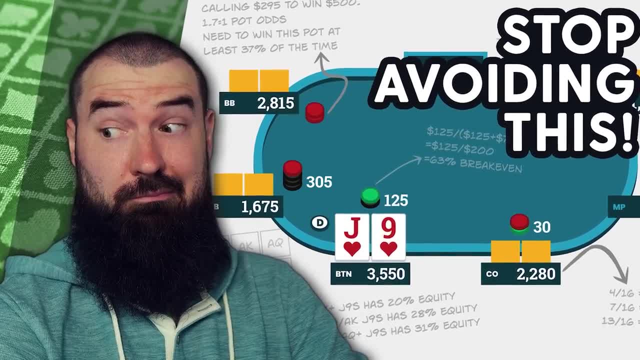 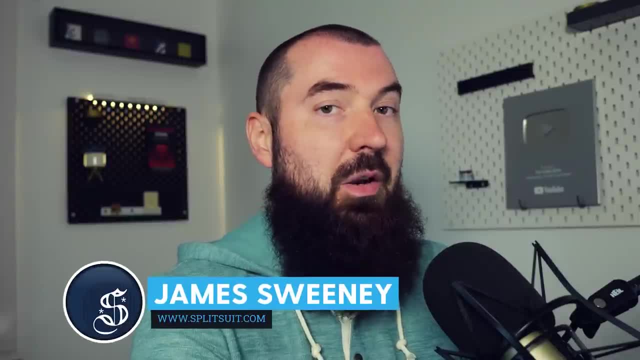 started. Good morning, how are we doing today? My name is James Sweeney, aka Splitsuit, And today I want to talk about some basic poker math with you and really make sure that you understand these principles because, honestly, every single solid poker pro that you know understands these things. 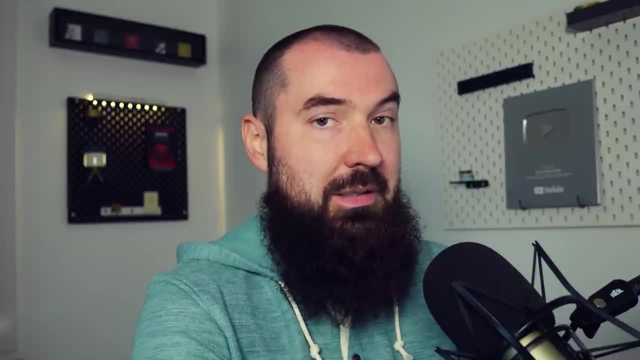 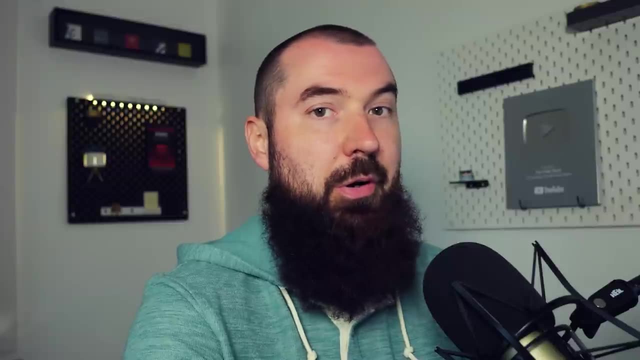 and most of the time is doing at least these basic calculations at the table, So let's fire right into it. The first concept we're going to talk about is pot odds, and pot odds are extremely simple. If you've been around poker at all, you've probably heard this term: a tremendous amount. 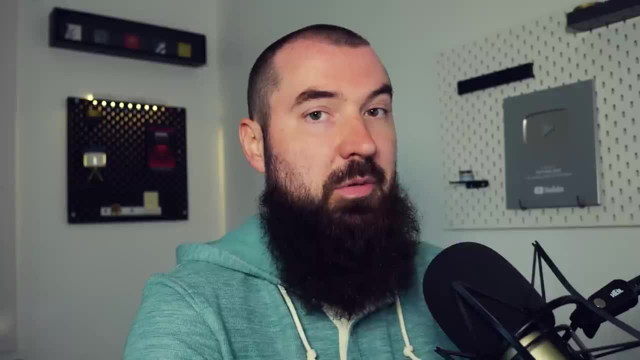 But a lot of poker pros are really good at it. So let's get started. Let's get started. players may throw the term around, but not necessarily be able to define it or calculate it all that easily, So let's go through a quick exercise together. Alright, so this is directly. 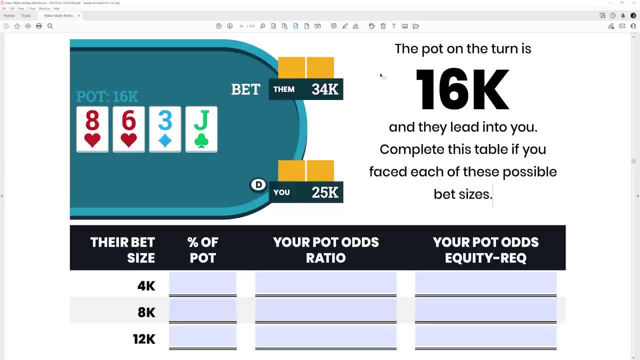 from my prefop and math poker workbook. And here's the situation: You're on the turn with a 16k pot, your opponent bets into you and you're going to do some general calculations of pot odds down below and pot odds. in case you're looking for a basic definition, simply compare the size of the. 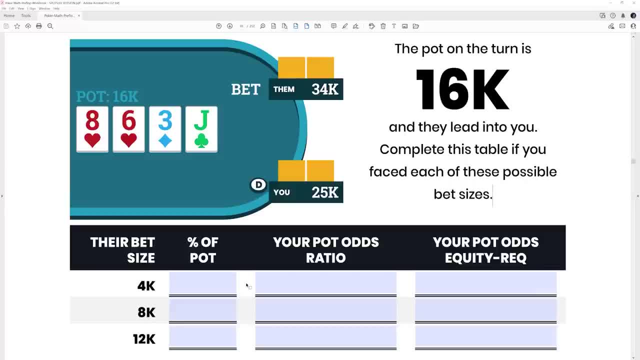 bet you have to call to the size of the pot. They are a mathematical expression of risk and reward That can then be used to make better plays, both preflop and postflop. So pot odds are offered anytime you face a bet, face a raise, it's regardless of what your overall cards are. 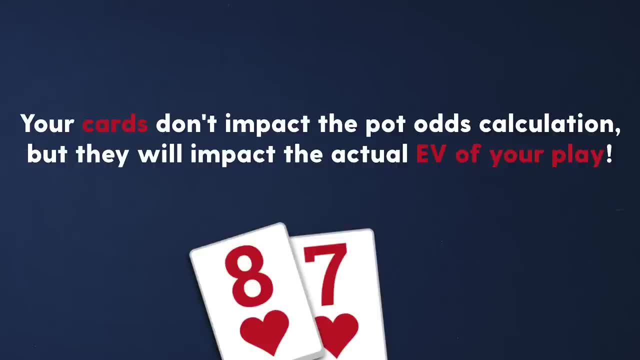 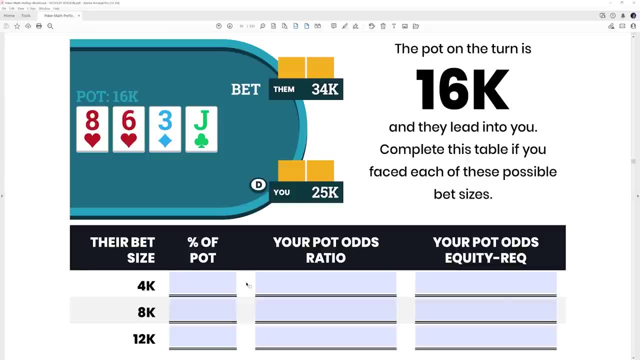 those don't impact anything. So if you're ever facing a bet or raise, you are getting pot odds. If you ever make a bet or raise, you are giving your opponent pot odds. So let's just burn through these real quick And if you are familiar with pot odds, maybe pause here real quick. 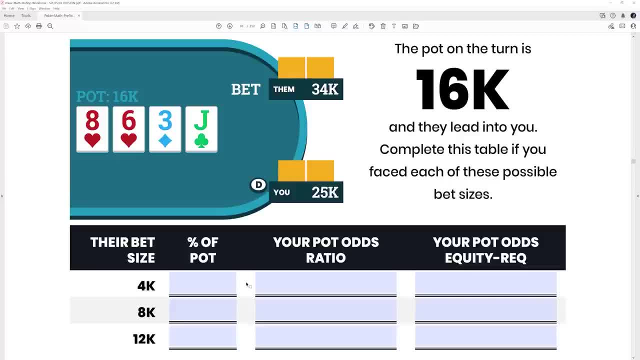 do the basic calculations, come back and make sure you did everything right. But here's the spot again: 16k in the middle, your opponent bets for 4k. So the total pot right this moment would be 20k right: 16 starter plus the 4k bet from them. 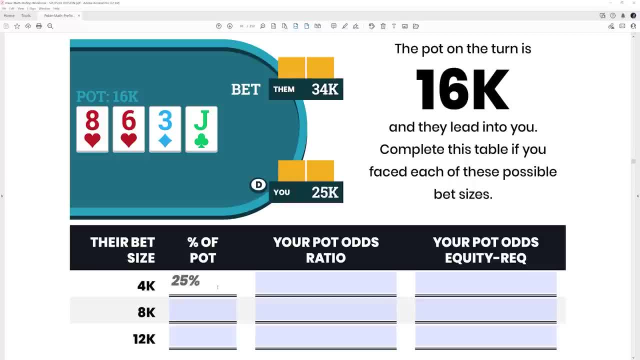 So the percentage of pots that they are betting right there is 25%, because they're betting four into 16, so one fourth. Your pot odds at that point are going to be five to one, And that's because, if you're thinking about what you're risking, 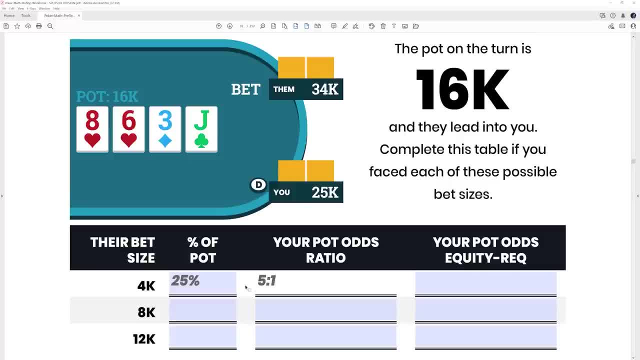 you are risking one unit, so the 4k unit. And what are you risking that for? You're risking that for five times that. the 16k in the middle plus their 4k bet equals 20 in the middle. so you're risking one unit to win five units. That's the way that I would think about pot odds. 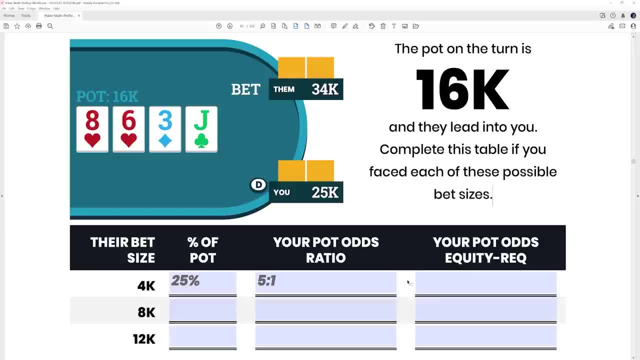 And I think if you're looking at ratios, that's the best way to think about them And if you're looking to understand what your equity requirement is, based upon that ratio, it's always risk divided by risk plus reward. So, in this situation, one divided by one plus five, or one over six, or 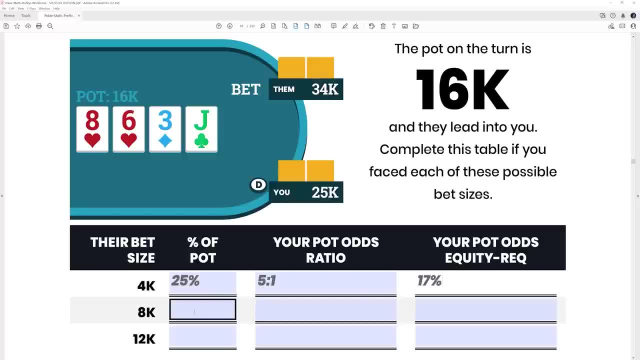 roughly 17%. Moving on to the next situation where our opponent bets 8k again into a 16k pot, they are betting at that point 50% of the pot. So you're risking one unit to win five units. So 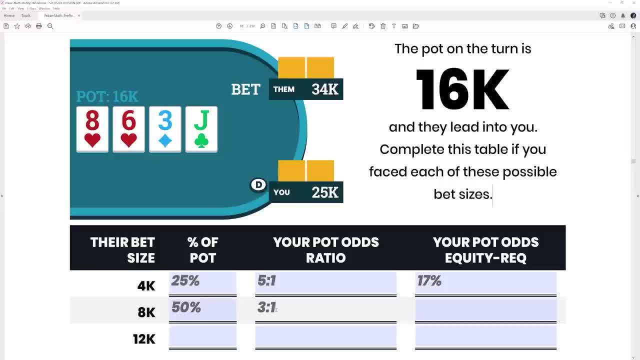 the ratio at that point would be three to one, right, Because we are risking our 8k call to win the 24k in the middle, the 16 plus their eight. So that gets three to one, And then the again. 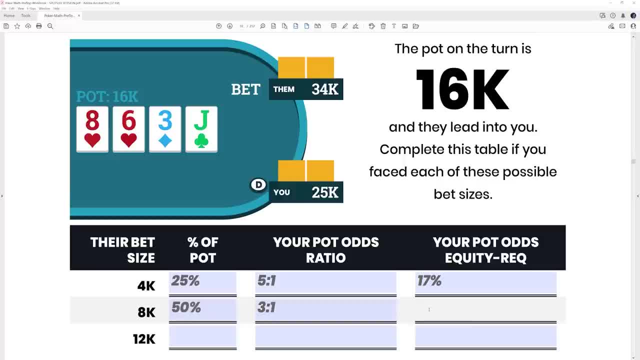 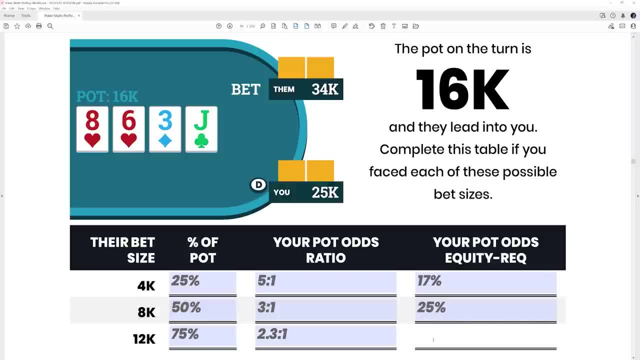 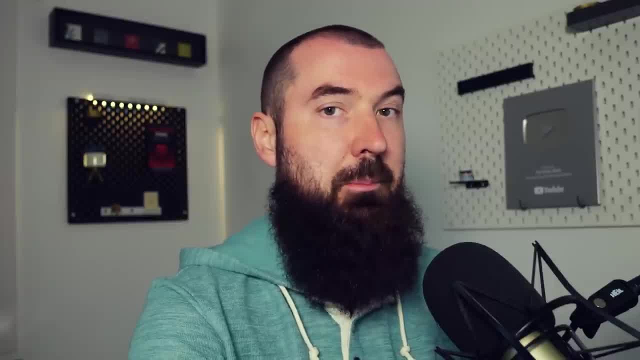 to one and the equity requirement to that point, one divided by 3.3 or roughly 30%, And because anytime you face a bet or face a raise, you are getting pot odds. It's very, very important that you have this formula understood And, honestly, you can memorize. 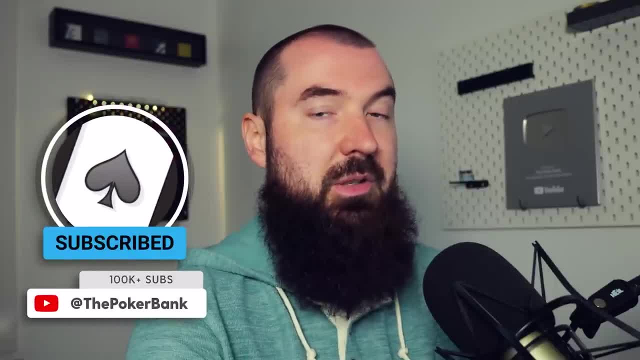 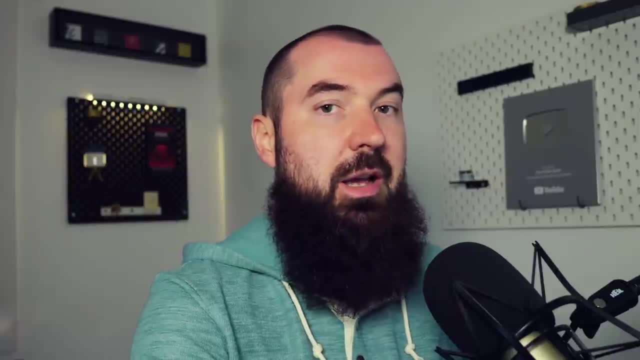 quite a few of these. If you just kind of memorize, okay, if I'm facing 25% pot or 50% pot or a hundred percent pot, that will really, really help you just kind of be able to estimate things in real time. You're not going to try to go down to a hundredth of a percent when you're doing. 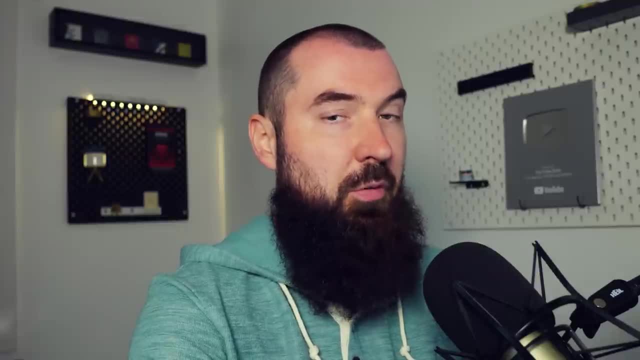 these kinds of calculations in real time. You're not going to try to go down to a hundredth of a percent in real time, Just kind of being close and in the ballpark is definitely going to help. And really the way that you want to look at this is you say okay, based upon the pot odds. 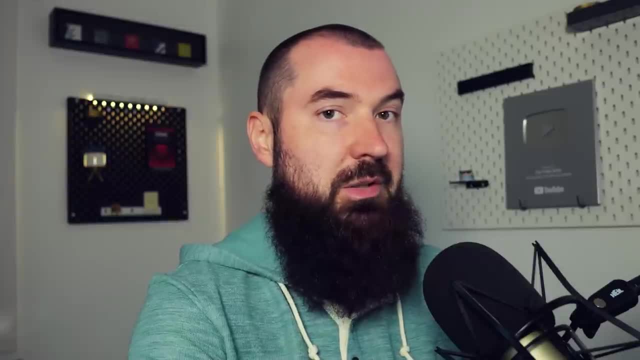 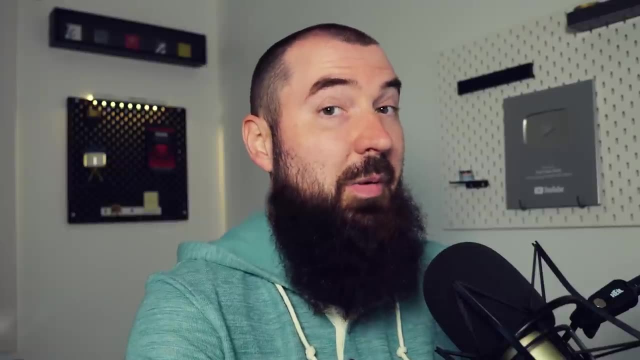 what is the equity requirement that I need right this moment in order to justify continuing? If you think your hand has that much equity, continue. If not, maybe not, but you could always at least consider a raise Hint. The next concept we're going to talk about is called. 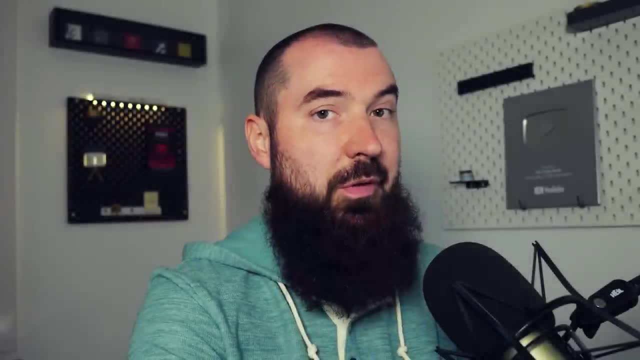 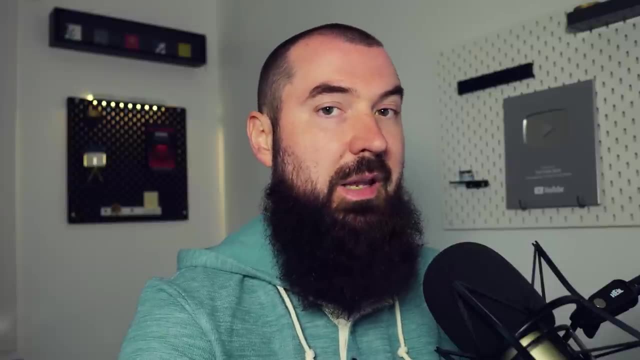 breakeven percentage. This is extremely important and also very simple to calculate and understand. So, unlike pot odds, when you're making that calculation, when you are facing a bet or a raise, breakeven percentage looks at times when you are actually the one making the bet or 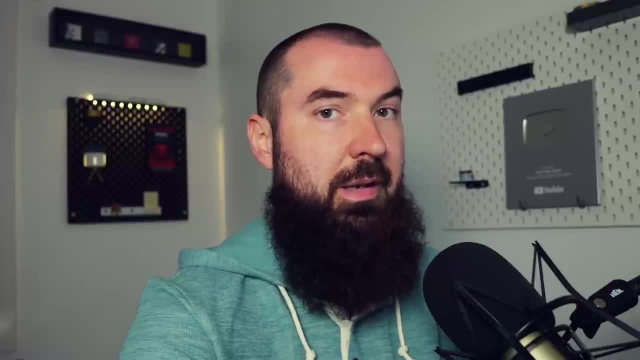 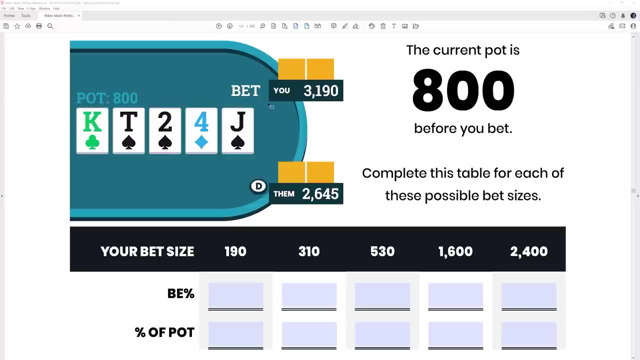 the raise. So let's flip back to the workbook and go through another example together. So we have kind of a similar situation. We have a spot, the pot right this moment is 800 bucks. this time You are the one betting and you're going to calculate the breakeven percentage based upon a couple of 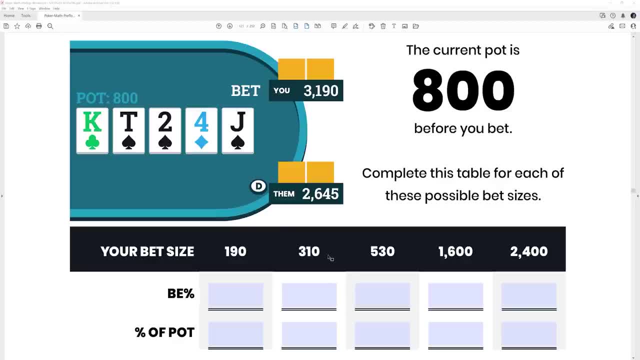 different bet sizes. So let's first start by talking about the 310 bet size, and this is roughly 40% of the pot, And then we have to calculate the breakeven percentage as well, And if you wanted to be very, very specific, you could go ahead and calculate the breakeven. 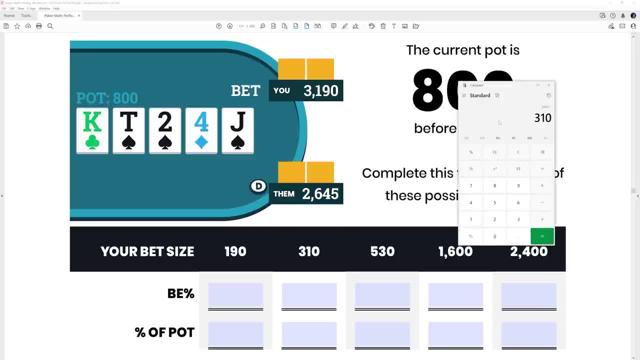 percentage based upon a couple of different bet sizes. So let's first start by talking about the 310 bet size And if you wanted to be very, very specific, you could just fire up a calculator. say 310 divided by 800.. That's going to be the percentage of pot, which is roughly 39%. 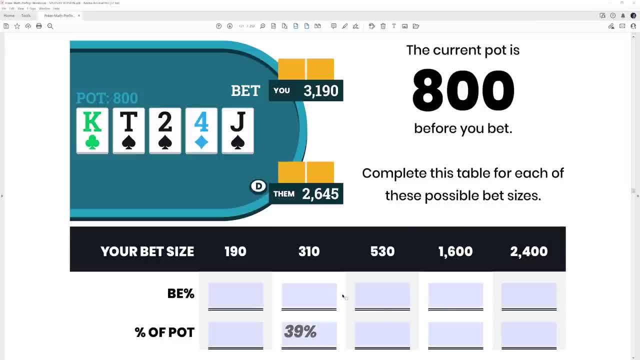 Just round it there, make life easy, And then the breakeven percentage is going to be again that risk divided by risk plus reward number, So 310 divided by 310 plus 800, or you can use my spreadsheet easy calculator that I have available for free. Leave a link. 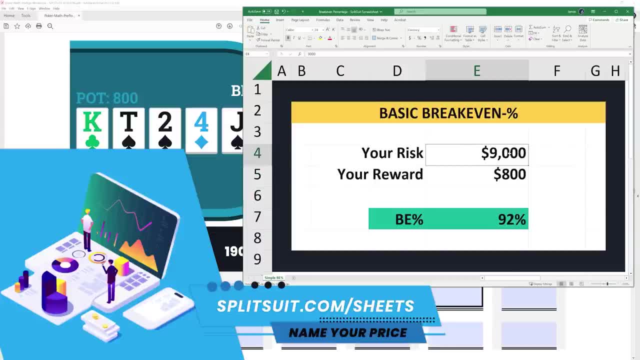 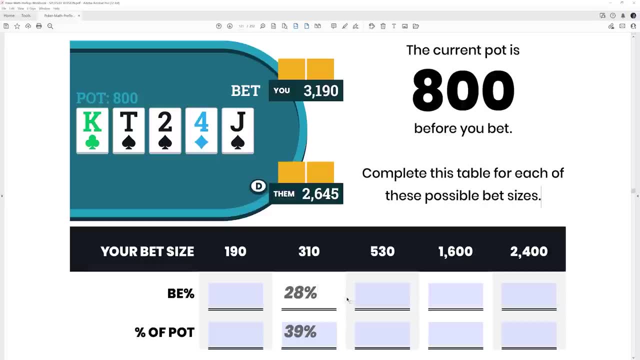 for that in the description box. The reward is 800.. The risk is going to be 310.. And the breakeven percentage comes out to 28%. And again, you can proof all of that out by using that formula: risk divided by risk plus reward. All right, while we're here, 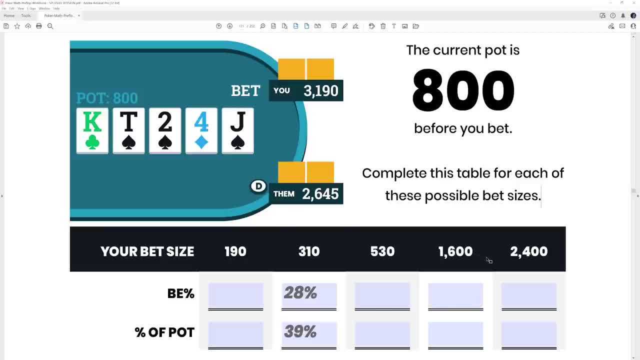 let's do another example on this page. Let's look at a $1,600 bet, aka a 2x over bet, in this situation. Well, we're betting 1,600 into an $800 pot, So we know that's going to be 200% pot. 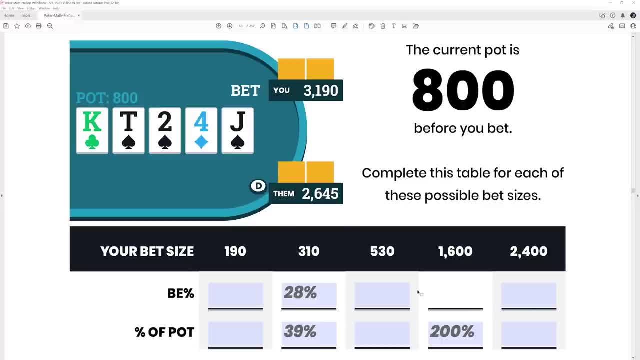 Perfect. And then the breakeven percentage again: risk divided by risk plus reward, or 1,600 over that. 1,600 plus 800 gets us a breakeven percentage of 67 or two thirds. And if you're looking at these two numbers and you're like: okay, I understand how to calculate. 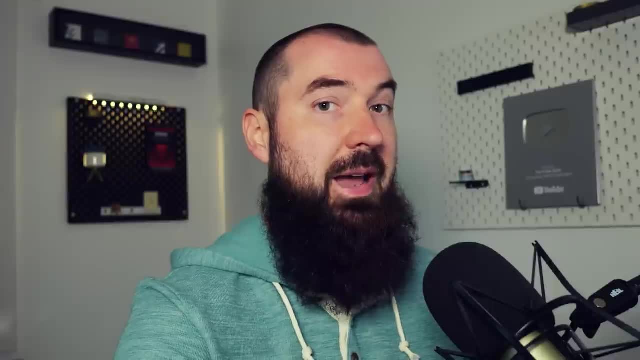 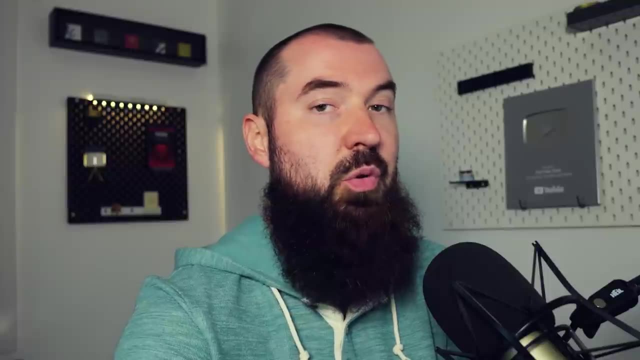 the breakeven percentage. but what the heck do I do with that number? That is going to bring us to our next concept: auto profit. So auto profit simply compares how often you think your opponent's going to fold to the required amount of folds from that breakeven percentage. So if your opponent is 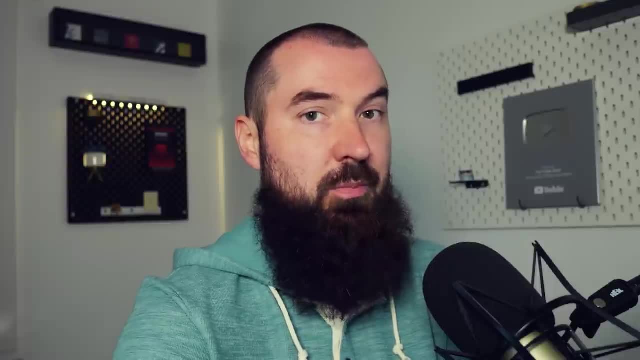 folding more often than the required breakeven percentage, you're going to be able to fold more. they are folding too much And, as such, you can make an auto profit by betting any two cards, which is great, especially when you're trying to find extra bluffs in your game. 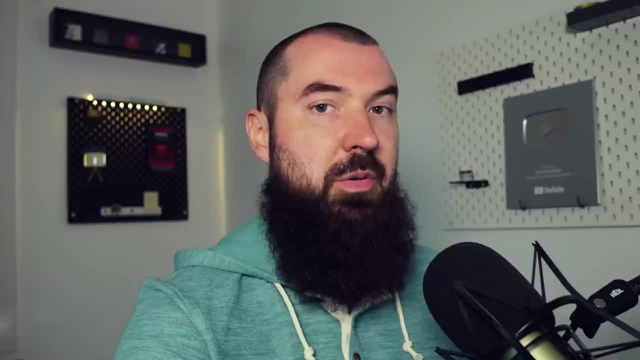 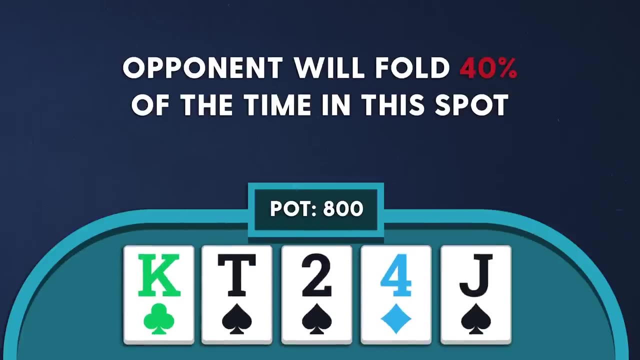 both pre-flop but especially post-flop. All right. So if we flick back to the workbook and try to apply this, let's just say: for whatever reason you think, your opponent is going to fold 40% of the time when you fire in this spot. Don't worry about what assumptions went into that, Just. 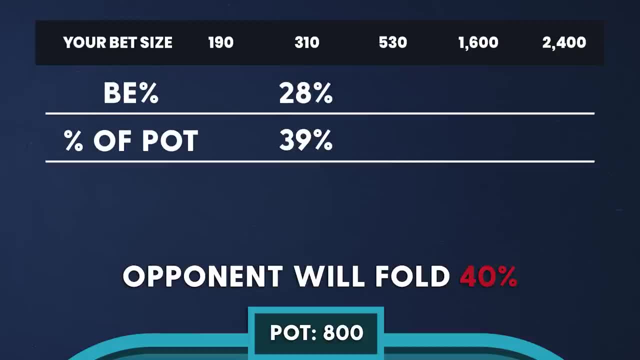 take the number for a moment. So when you fire for 310,, the breakeven percentage is 28%. You think they're actually going to be folding 40% of the time. So 40, is higher than 28. And as such, it is auto profitable to fire in the spot. 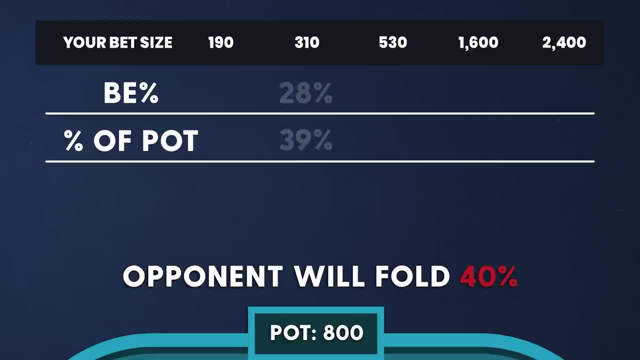 which means you should be firing more and more bluffs. However, when you bet 1600 or 2x over bet it, notice that the breakeven percentage is 67%. You still think they're folding 40% And, as such, that is not going to be auto profitable Now, in the real world, obviously. 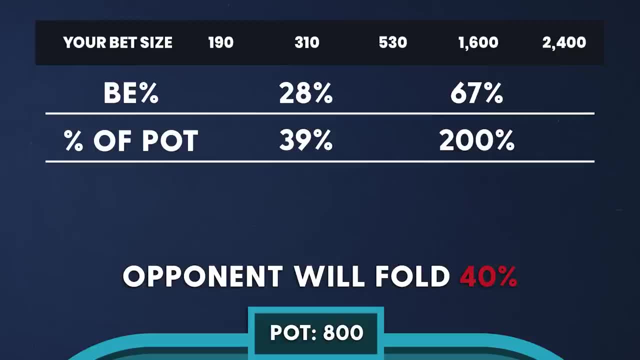 most players are going to have some level of elasticity, which means they're going to continue differently against these two numbers. right? If you bet 310 versus 1600, maybe they continue more often against 310. And if you bet 310, you're going to have some level of elasticity against. 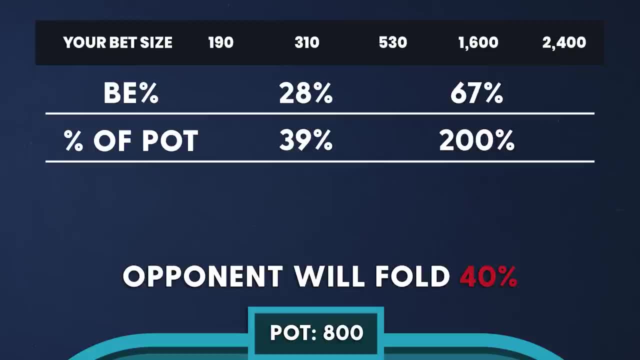 1600 and less often against 1600.. So while you still will have the exact same breakeven percentage based upon the size, the actual continuance frequency or folding frequency that you're comparing for auto profit numbers is going to or can possibly change, So keep that in mind when 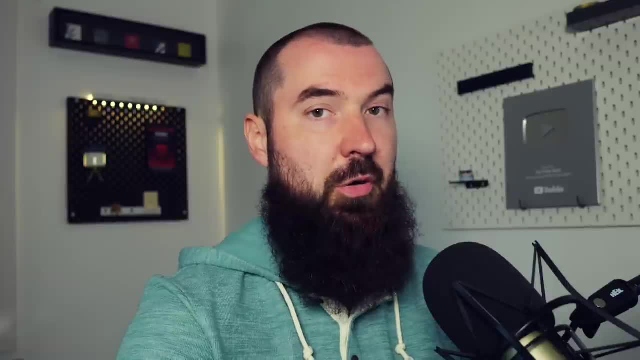 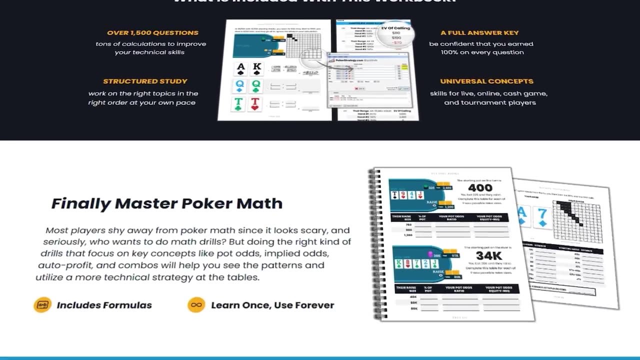 you're doing a real world analysis And for what it's worth. there are actually auto profit explorations within this workbook. I'm just going to gloss over it for now because I think you have the big picture idea, but if you want more work, definitely make sure to check out the workbook. 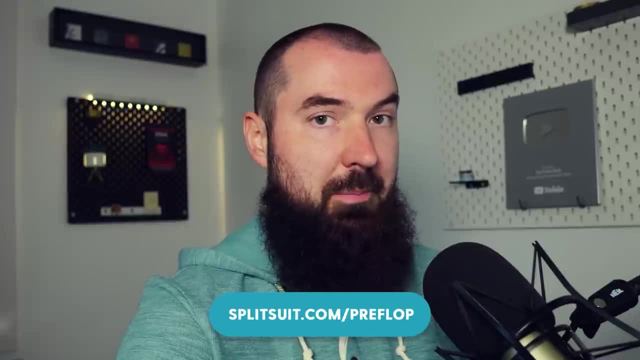 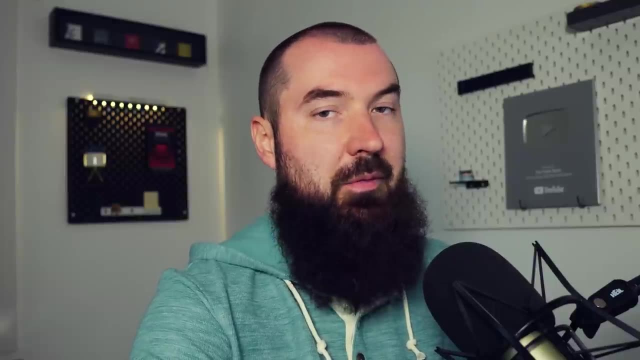 splitsuitcom, slash pre-fop to learn more and pick up the next one. All right, the next concept that pros are definitely keeping track of in real time- maybe not exactly perfectly, but they minimum have a rough count going on- are combos and also thinking about blockers and how they relate to combos. So combos, essentially. 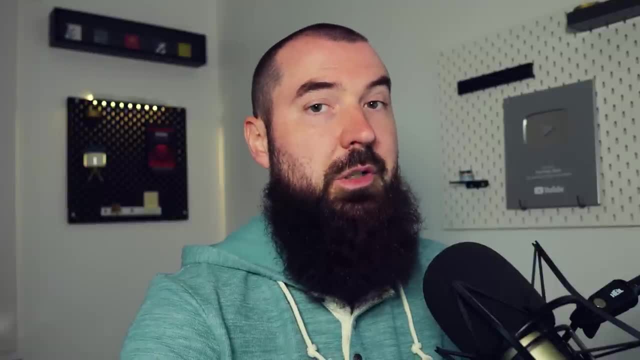 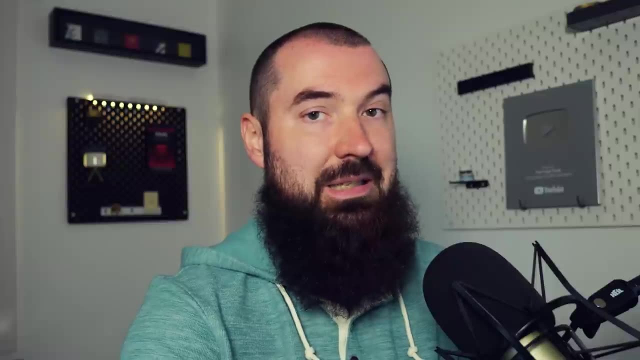 count how many different ways a certain hand can be made. So, for instance, if you're trying to count how many combos of ace king suited there are, there are four: ace king of hearts, ace king of spades, ace king of clubs, ace king of diamonds And then blockers. essentially look at any known. 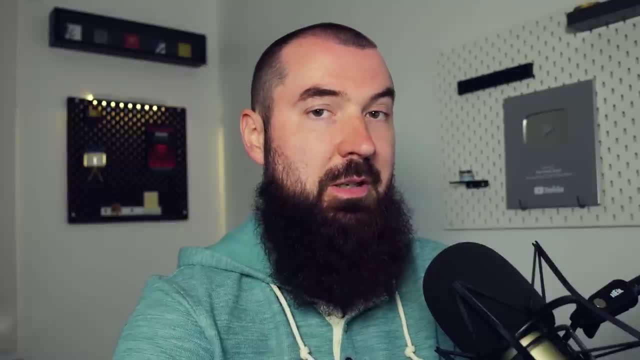 cards or cards you can visibly see, to see if they're going to be able to do a good job of any combos need to get removed. So, for instance, if we're still looking at ace king suited example, let's just say that you have the ace of spades. you have ace of spades, queen of hearts. Well, 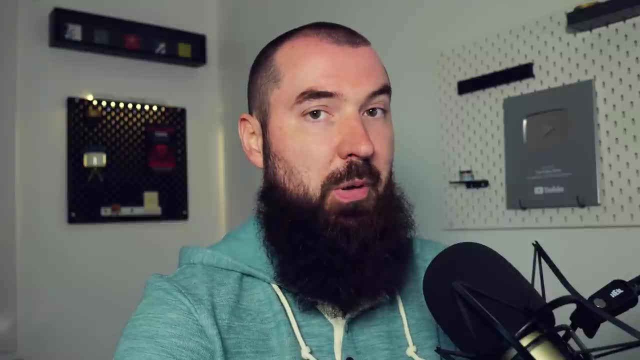 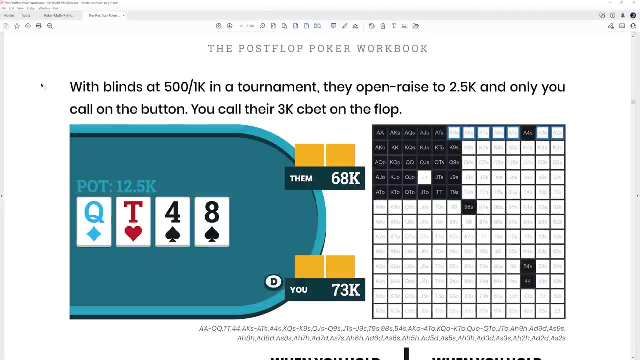 based upon that. your ace of spades now makes it impossible for your opponent to have ace king of spades. That blocks out those combos. So if we flip over to a workbook, this time we'll use the post-flop workbook instead of the pre-flop and math one. This is a combo exercise. So since you 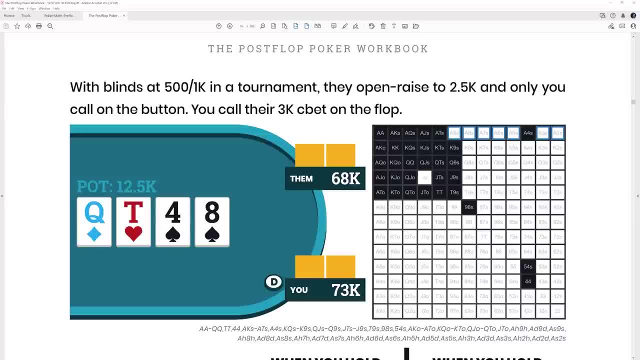 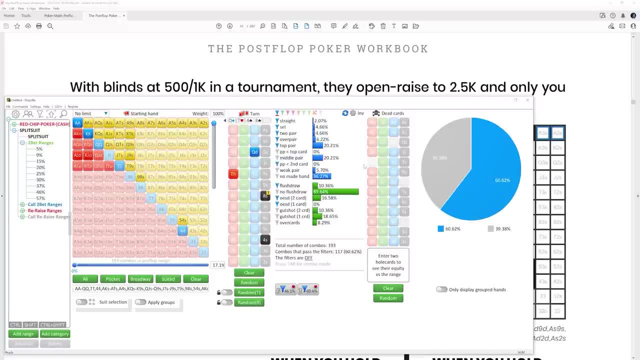 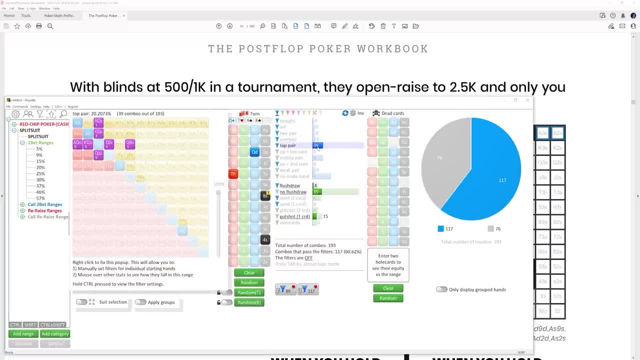 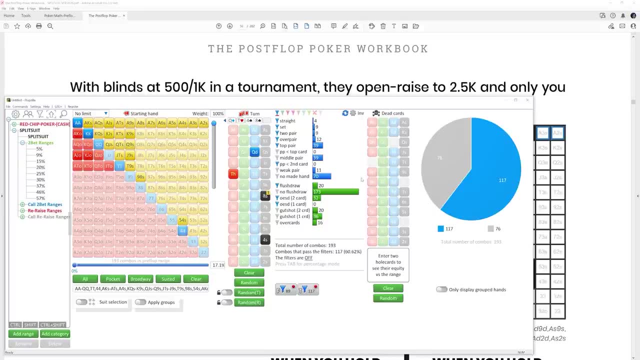 mode, just hit the tab key. And now all of these numbers are going to be looking specifically at combos instead of being in percentage or stat form, And one of the things that pros are especially keeping track of throughout a hand, or at least trying to keep a rough idea of, are the number of 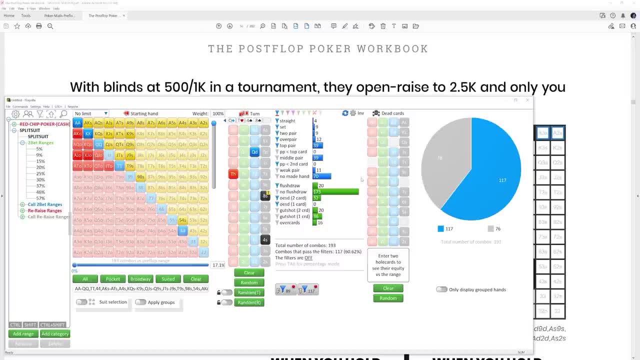 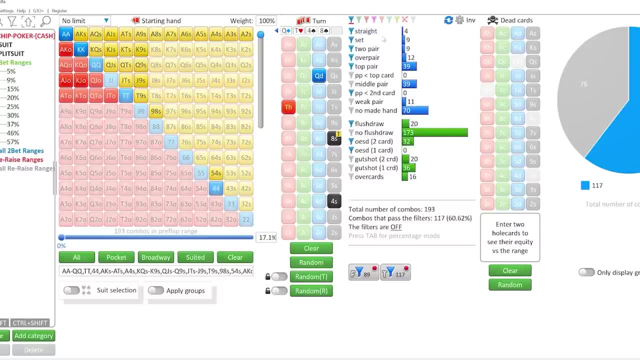 combos of really, really strong hands, their opponent can have right this moment. So in this situation, if we look at really strong hands, let's just say over pairs or better, notice that there simply are not very many of these, especially when compared to the overall number of combos. 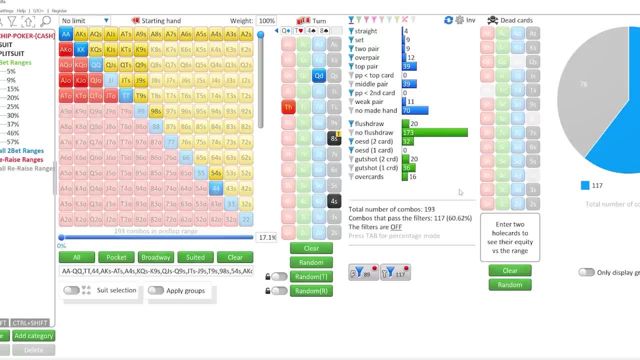 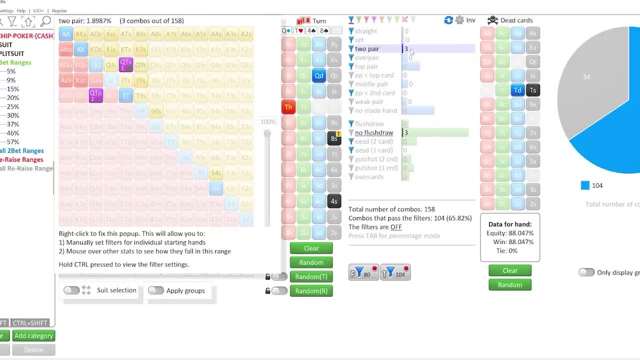 that got to this street at roughly 193.. And this is all before we factor in blockers, by the way. So let's just say, hypothetically we had pocket tens in this situation. Well, notice, that's going to do even further removal and block some more of those strong combos. Now your opponent really. 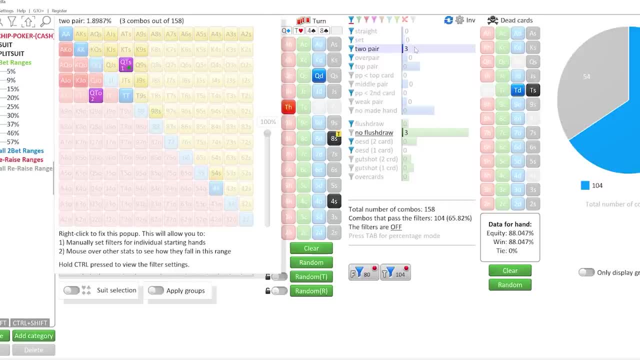 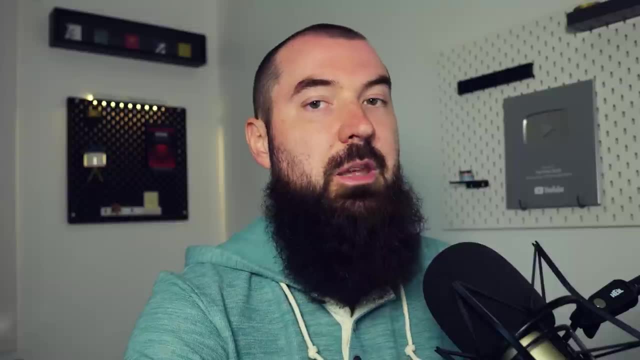 can't have a set of tens. All of a sudden, their two pair combinations are massively degraded, And that of course means that they have less and less super strong hands in their range right this moment. So by keeping track of the rough number of really nuttish combos in your opponent's range, especially if the density of 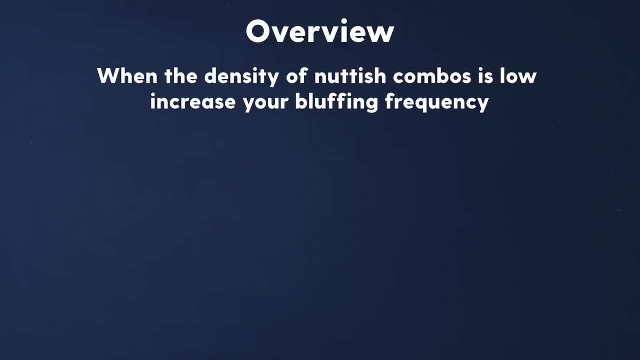 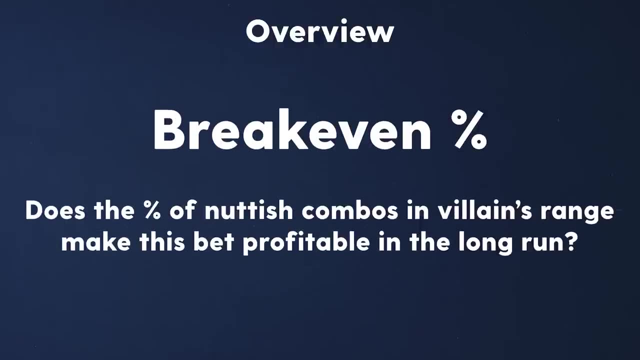 those really strong hands gets very, very low compared to their overall range. that can be a great situation for you to start bluffing a tremendous amount, And this is how you can start tying the concepts together. You go back to your breakeven percentage. you think about: 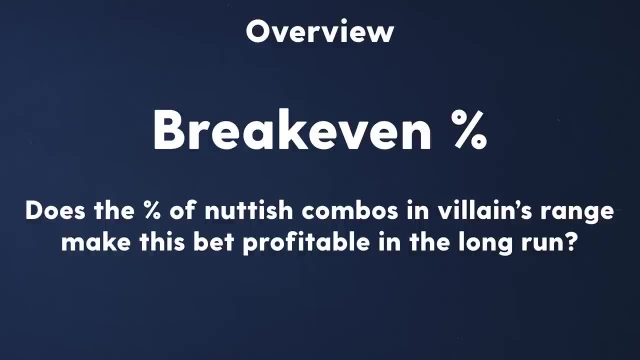 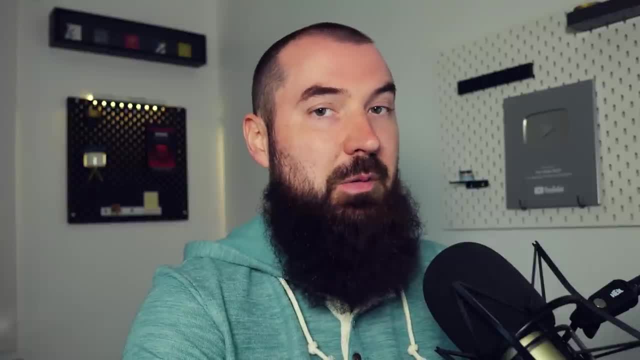 auto profit. is your opponent going to fold often enough? Hint, this is how you can mathematically start looking at that and finding that actual fold frequency from your opponent. This is exactly how you can start tying those concepts all together And the final. 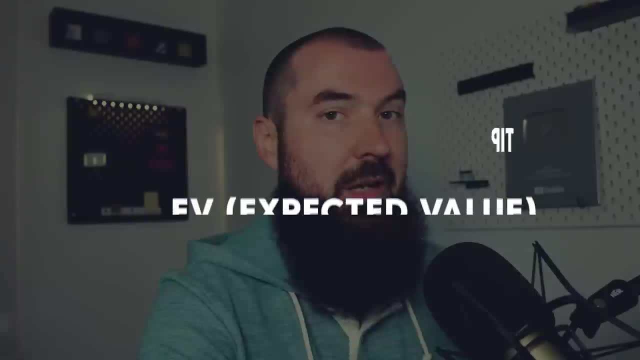 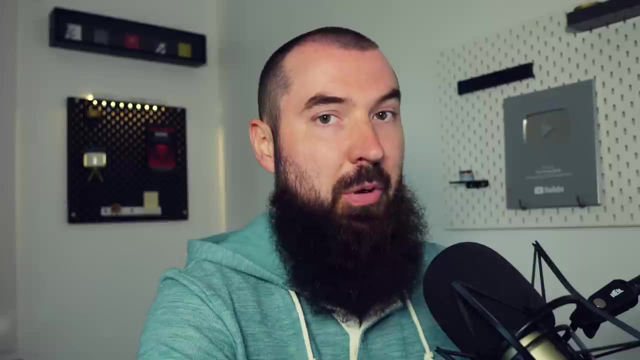 concept that I want to touch on today that all poker pros are keeping track of is EV. Now, almost no one is calculating this to the dollar by any stretch of the imagination in real time, more just eyeballing it and trying to make sure they take as many plus EV situations as possible. 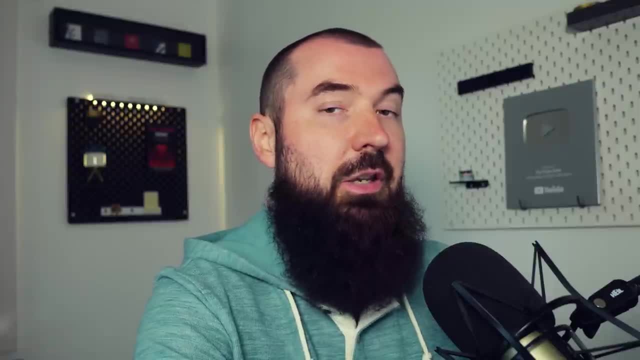 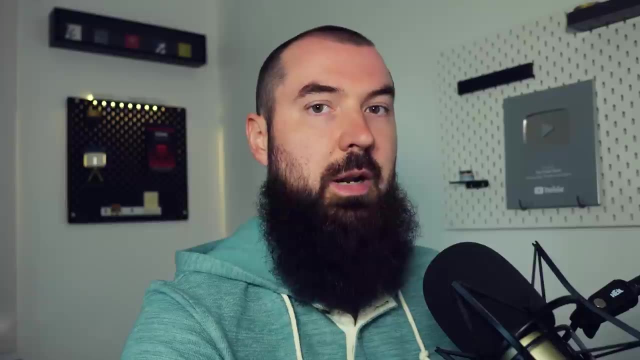 aka things that are expected to net them money in the long run, and trying to remove as many negative EV decisions from their playbook as humanly possible. Again, things that are going to net them losses in the long run. All right, so let's flip over to another example from the. 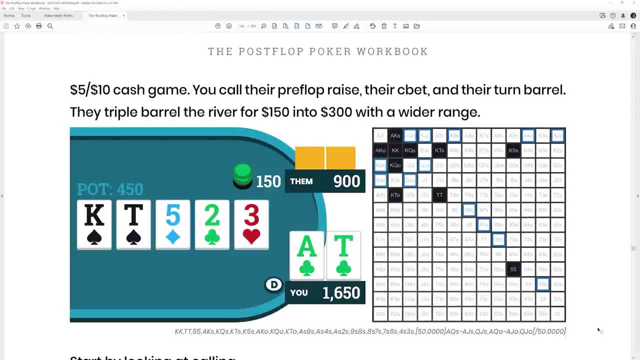 post-flop workbook. This time we are on the river with, let's say, a $100 pot. So we're going to be taking a $300 pot and we're going to be taking a $200 pot, and we're going to be taking a $100 pot. So we're going to be taking a $100 pot and we're going to. 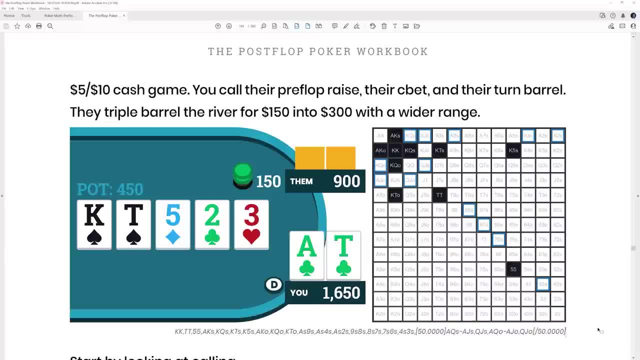 taking a $100 pot and we're going to be taking a $100 pot. So we're going to be taking a $100 pot. So there's currently $450 in the middle and we have second pair and we're thinking about turning. 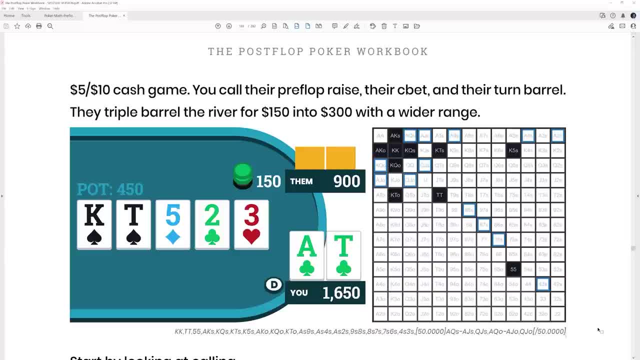 it into a bluff shove. So what do you think the EV might be? If you've never worked with EV before, this is going to be pretty much impossible to answer. but if you've done a couple of EV calculations, take a quick eyeball estimate and then let's run through the math together. 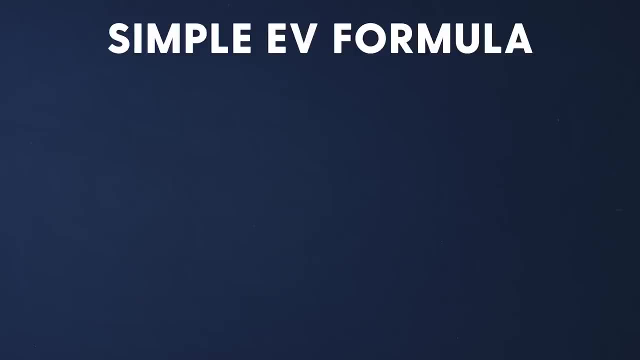 So the basic EV formula, if you've never seen it before, is how often you win multiplied by how much you win when you do in fact win it, minus how often you lose times- how much you're going to lose the times you do in fact lose it. And this can be expanded out greatly, depending on all the 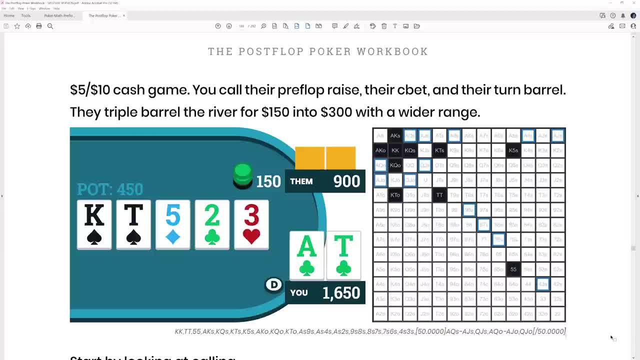 different outcomes that can possibly happen. Now in this situation, if you think about our bluff shove here, what are the possible outcomes that can happen? Well, we can shove our opponent folds and we win the pot, right that moment. We could shove our opponent continues and we win that. 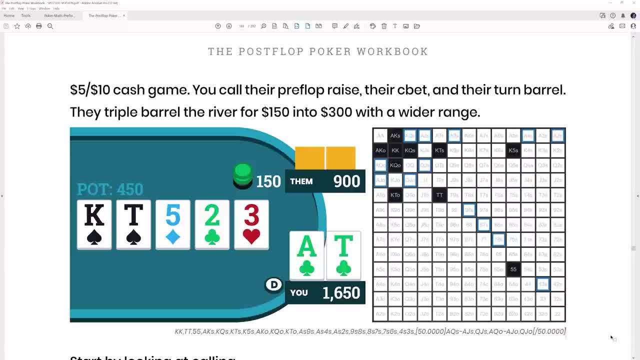 pot, or we shove, our opponent calls and we lose that pot. And since we're talking about second pair here, let's just make the basic assumption that our opponent is not going to continue with second best hands. So essentially, if we shove and our opponent calls, we lose. Doesn't matter if we lose. 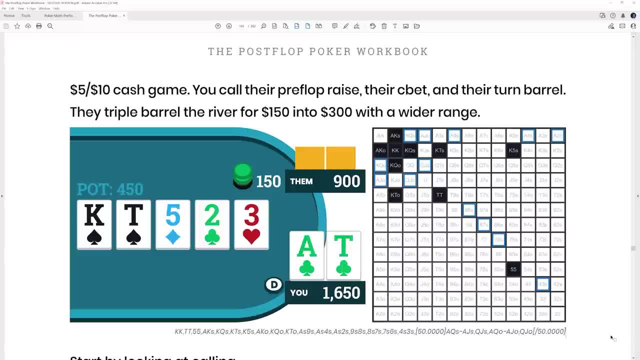 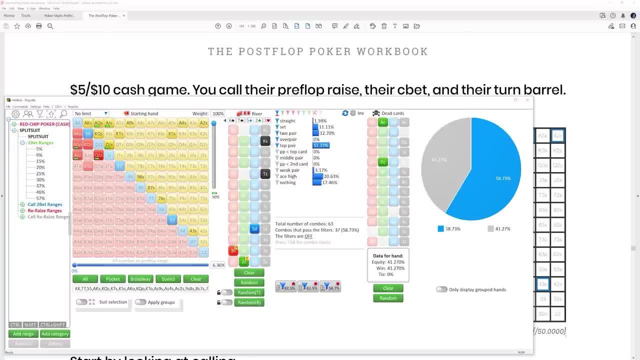 to top pair or if we lose to two pair. whatever it is, we're just going to make that assumption for the time being. So when we fill up everything inside of Flopzilla, here we are and we notice that if we assume our opponent is always going to continue with top pair or better, don't worry if 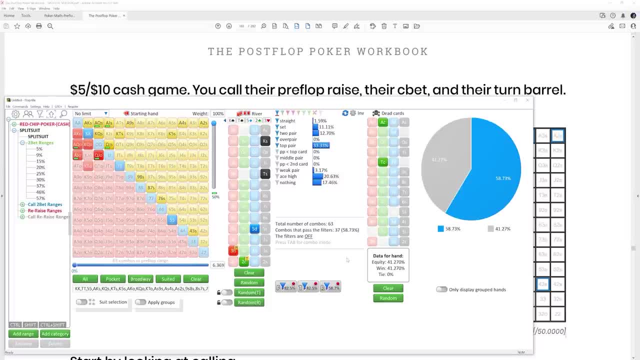 you agree with that or not? just work with it for the time being. that means that our opponent is going to be 9% of the time and thus fold the other 41% of the time, and then we can plug all that into a quick calculator. Now, of course, in real time you're not going to be able to pull out. 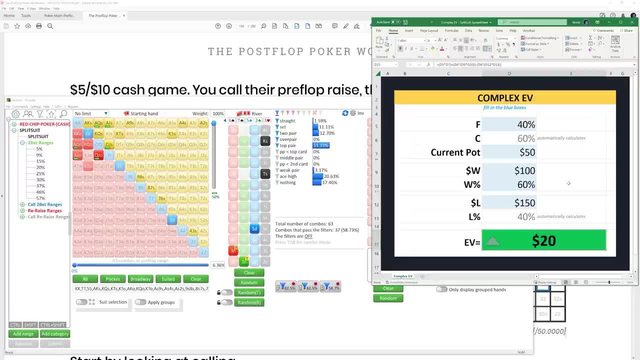 a calculator and actually do this. so the work or the idea is, is that by doing enough of this work off table, you can better estimate and eyeball this stuff in real time. And really that's what the best pros are doing: They're eyeballing it, they're estimating, they're saying okay, I think. 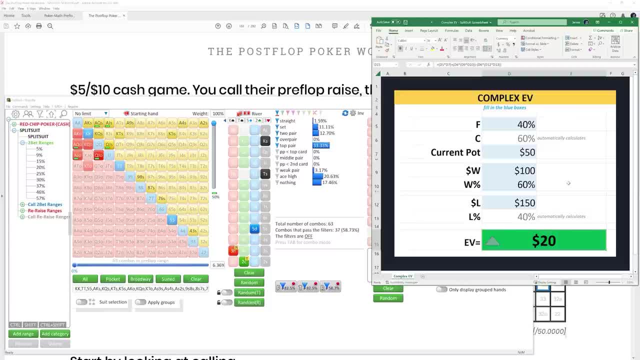 this is going to be plus EV, I think it's going to be super plus EV, or I think this is going to lose me money and, as such, it's negative EV, and I'd rather just not make that assumption Instead, because we could always just fold, facing this bet on the river. we don't have to. 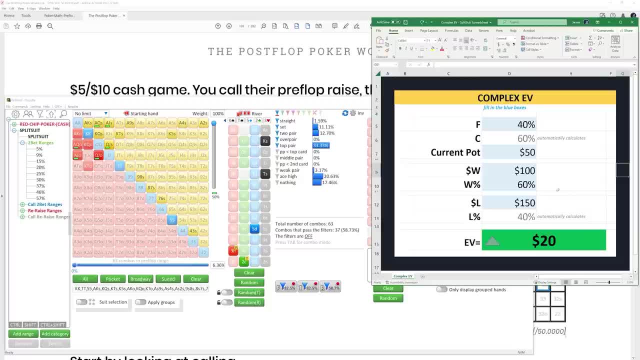 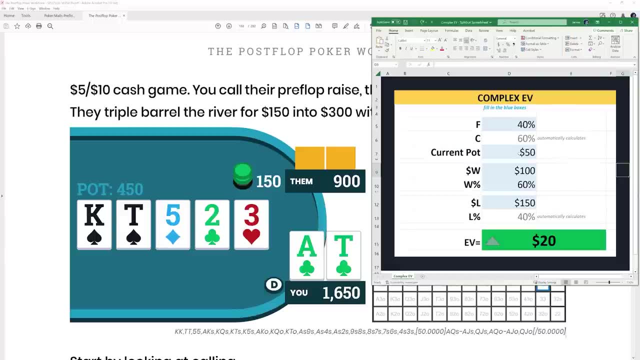 come along for a shove, All right. so let's take a moment and fill out the complete calculation so we can see what the EV of this shove is. Let's go back and let's look at a couple different numbers. So, first and foremost, how often is our opponent going to be folding right this moment? Well, 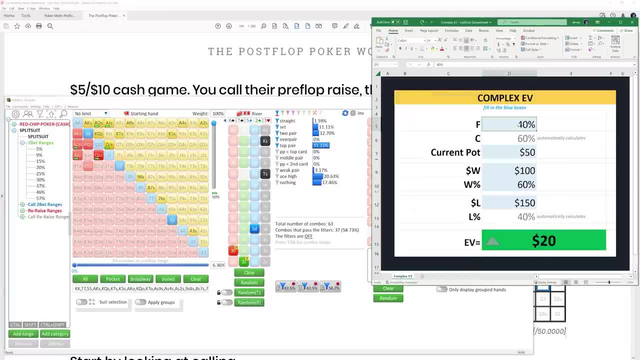 we just calculated that in Flopzilla it looks like they're folding 41% of the time. Fill this to 41, C will automatically calculate in the inverse. so 100% minus that number equals the C number. That's how often they're going to continue. 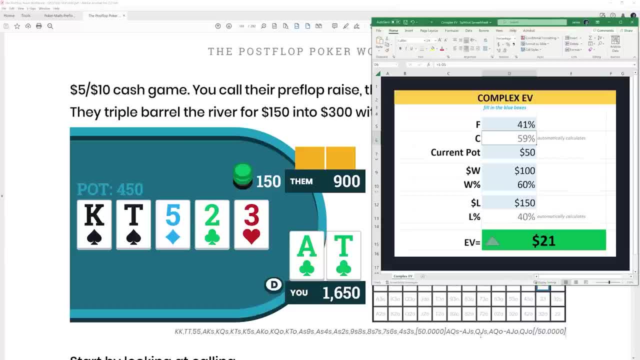 The pot right this moment is $450.. Perfect. Now, in this situation, we're expecting that when we shove and our opponent continues, we never win that pot. So because of that, we can just make the win percentage zero, which means that we're going to lose it 100% of the time when continued. 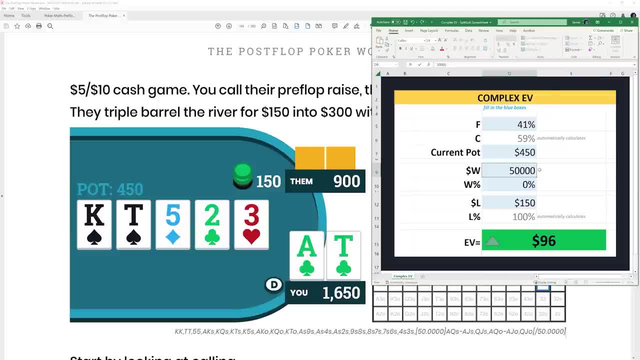 and, as such, what number you put in here does not matter. You could put 5 million or whatever number of zeros. It's not going to impact the EV because, again, you're never winning it, So it doesn't matter. What does matter, though, in this situation, because when we shove and get continues from. 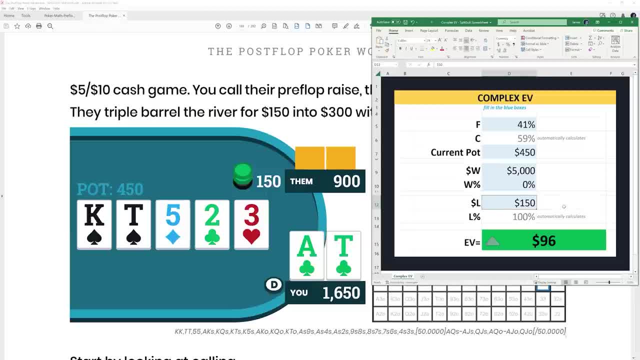 our opponent. we are never ahead is how much we're losing in those situations. So we would lose, since we cover our opponent. we would lose $900 plus their $150 bet. So we can just factor that in right here: $900 plus $150.. Cool, And you notice that our EV for this shove, based upon all, 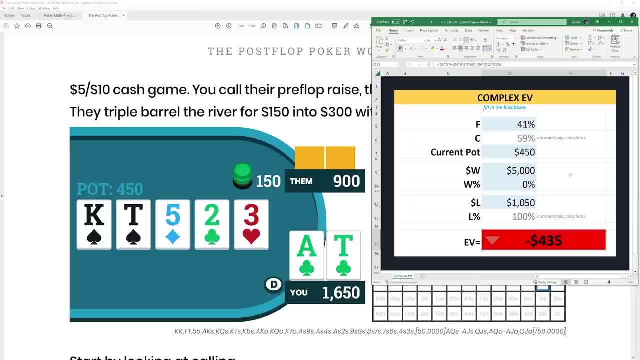 the parameters and assumptions is $900.. So we're going to lose $900.. So we're going to lose $900.. negative $435.. So not super great. And if your first thought with this is: well, congrats. I'm not a human calculator and as such, I can never do this in real time. I totally understand. 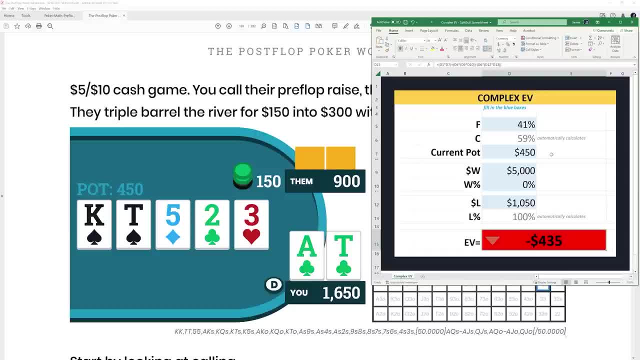 But you can eyeball this right. You can just say, okay, well, my opponent's folding less than half the time. When I do pick it up, I'm picking up just the $450.. I'm risking much more than that. 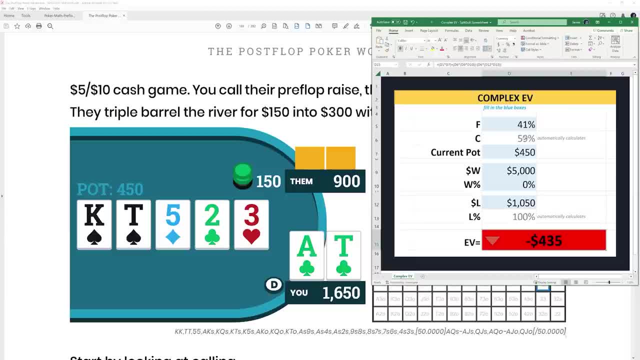 And when I get continuance, I lose it 100% of the time. They are continuing a decent chunk and, as such, you know it's going to be negative EV. Maybe you can't tell that it's going to be negative $435.. Maybe you can't tell that it's going to be negative $435.. Maybe you can't tell that it's going to be. 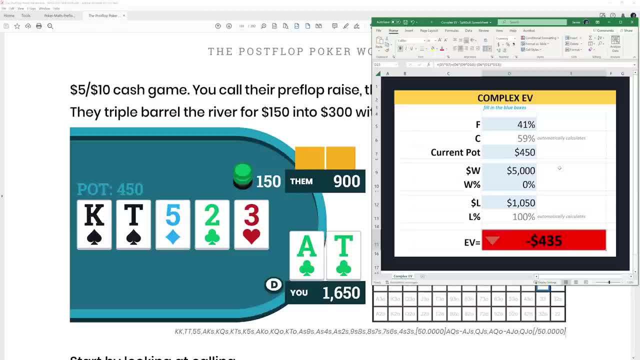 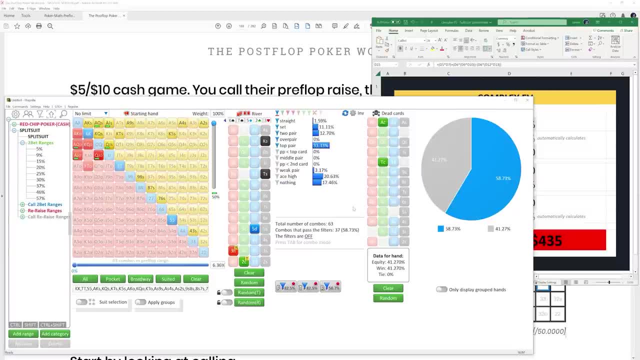 negative $435.. That's fine, But at least you can identify a negative EV situation. But what if we change things up just ever so slightly? go back to Flopzilla and think, okay, well, actually I think they're going to continue with fewer combos than that. I don't think they're going. 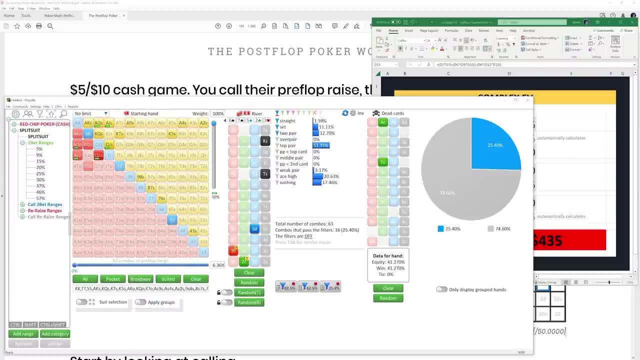 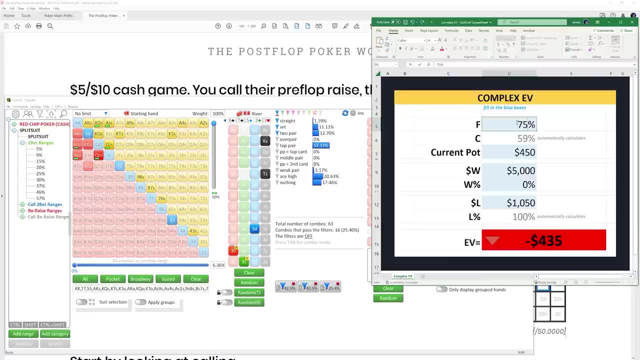 to continue with top pair every time. I think they're only going to continue with two pair plus. Well, now all of a sudden they're folding much more roughly 75% of the time, and that's going to change things at least slightly. So change this up to 75.. And now all of a sudden you notice 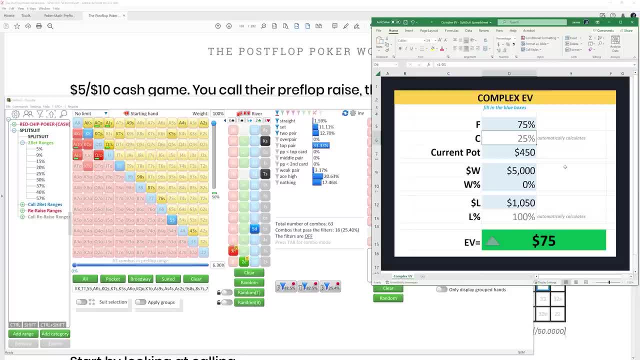 even though we're still losing $1,050, every single time we shove and get called. we're not getting called nearly as often And, as such, this is actually positive to the tune of 75 bucks, So no one's expecting that in real time. 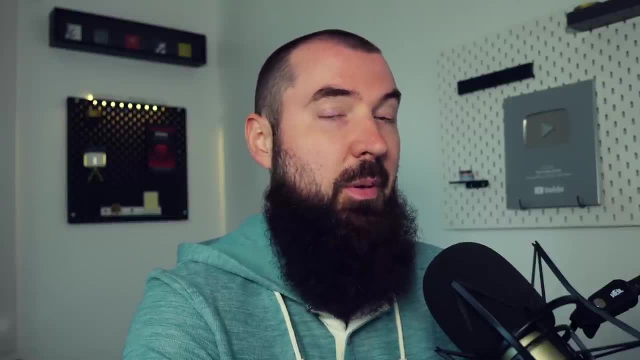 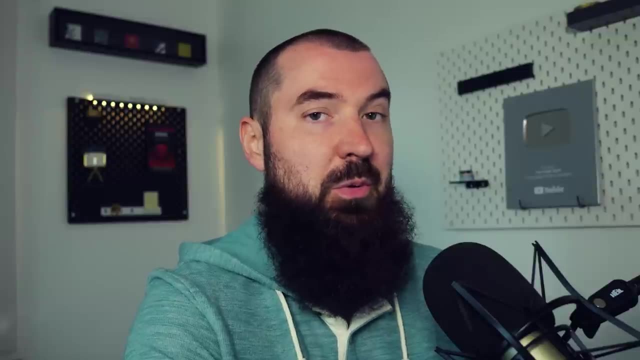 you're going to be able to calculate this as exactly plus $75.. However, if you can get better and better at eyeballing this, which is going to be done through off table reps and practice, it's going to be much, much easier for you to identify situations where your opponent is. 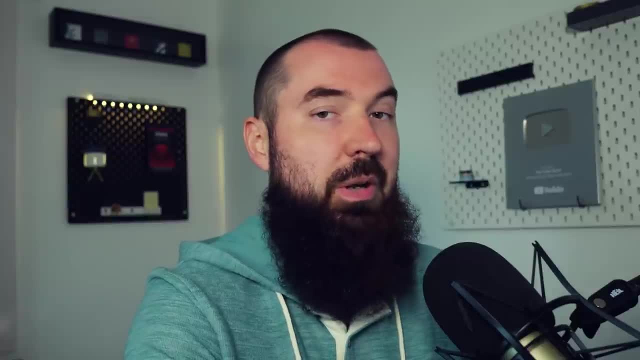 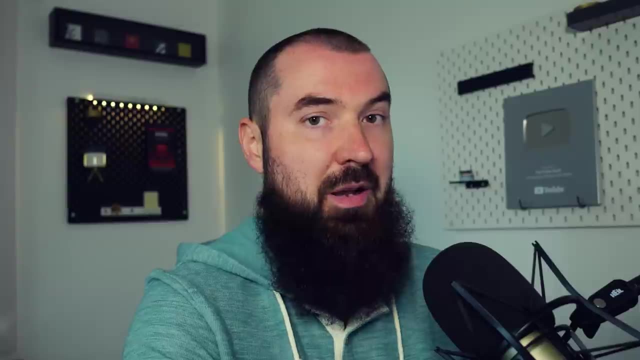 folding more often, you can find more bluffs. you can make sure you're deleting more negative EV plays from your playbook, both pre-flop and post-flop. But it's by doing this kind of off table work and understanding these big picture math concepts. 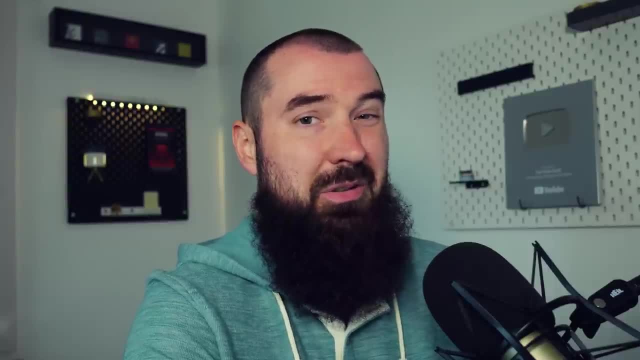 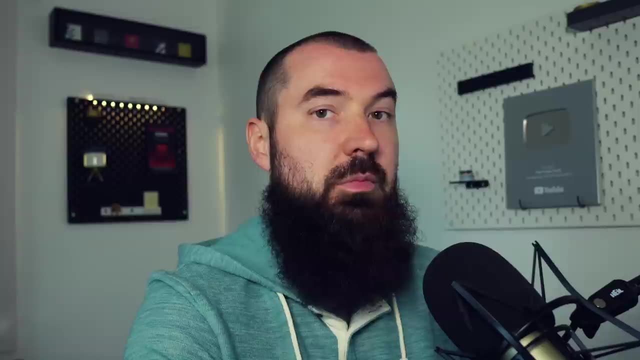 you can really start to piece together an entire strategy, rather than just kind of cobbling together whatever current strategy you have right at this moment that might not be working for you as best as you'd like. So again, all of these poker concepts are things that pros 100% know. 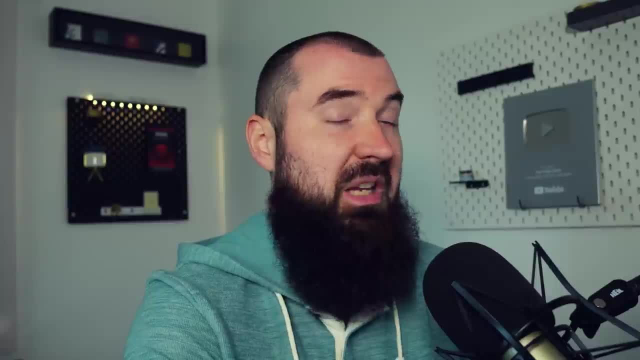 keep track of and are trying to do basic calculations in real time. Again, no one's expecting you to be pixel perfect, but at least if you can get in the ballpark and you're getting better and better when your opponents are in no way, shape or form, trying to.